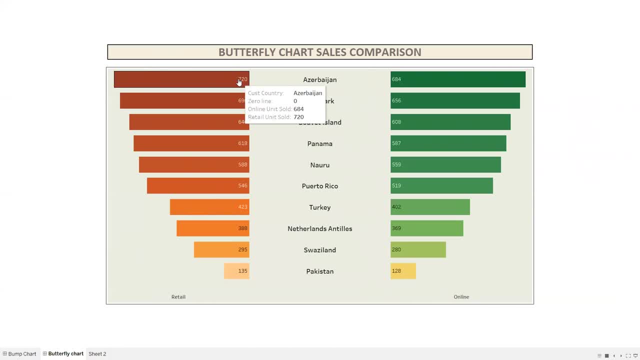 retail sales and the right side is the online sales. So it's actually comparing the sales channels, how the retail is doing and how online is doing for the same country. So this actually even useful for when you are doing the population, let's say how the male gender. 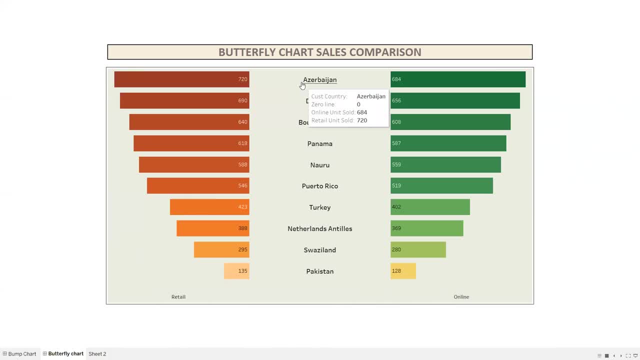 in which countries a male gender population and female gender populations, So that also we can compare. or else you can compare the product level, two different products, how they are comparing, as well As you can take the for one product, how the previous year sales and how the current. 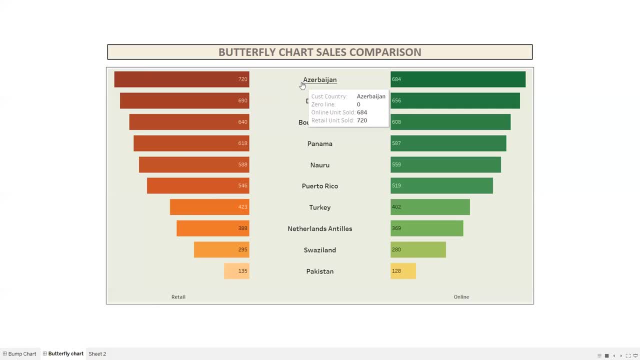 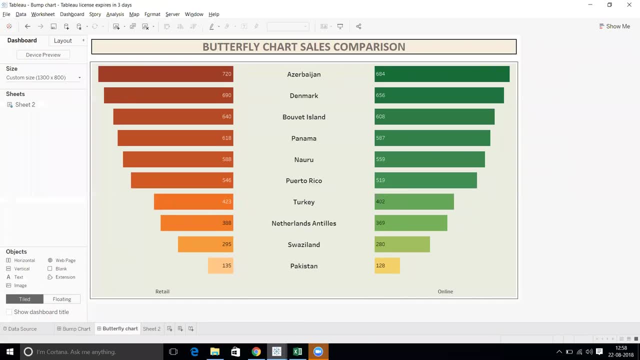 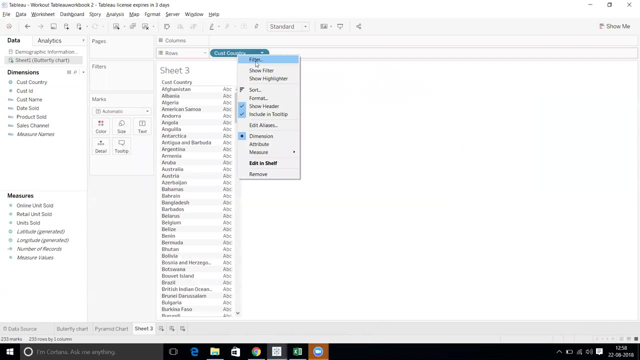 year sales is so that you can do in a butterfly chart, Okay, so let's get into our how to do this. I have a data set here, So I'm taking the customer country customer and I'll take only the top top 10 customers. 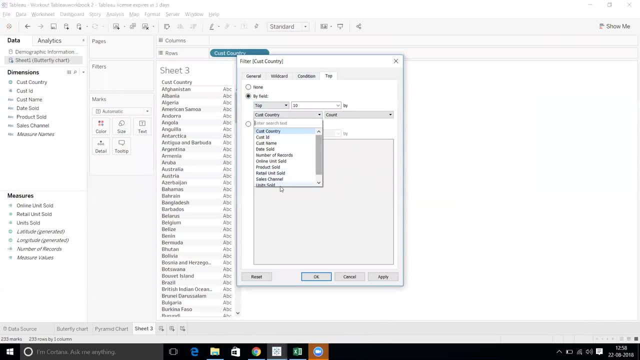 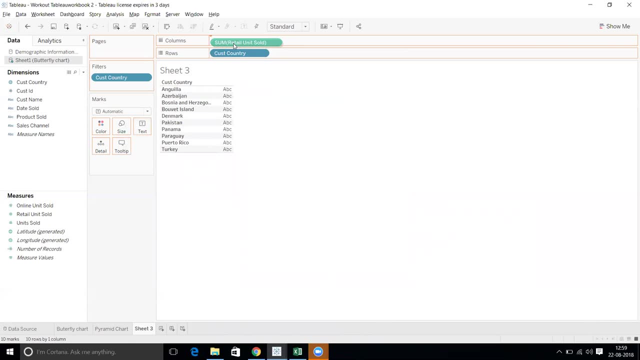 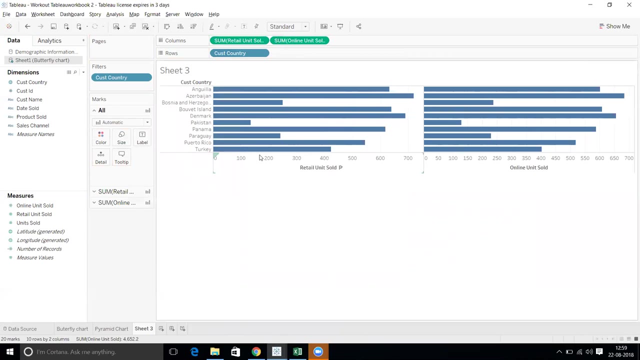 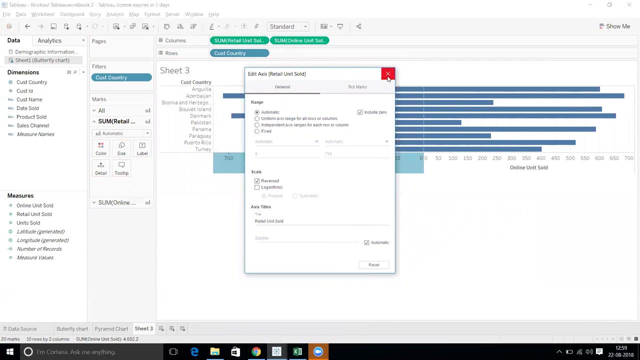 Top 10 countries based on the units sold. Okay, so next I'll take retail units sold And one more is online units sold. I'll put it in a reverse. Okay, fine, So now I need to sort this from top to bottom. 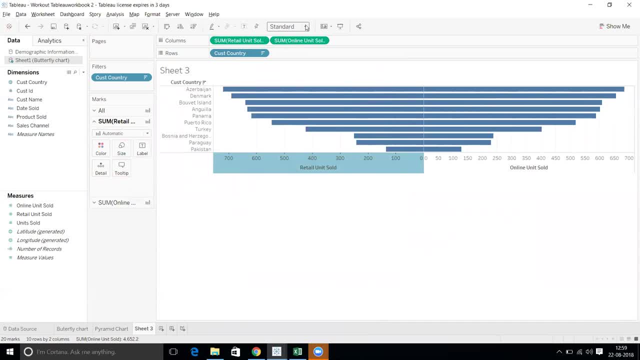 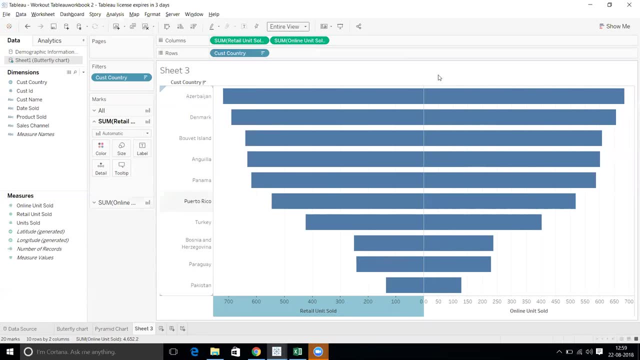 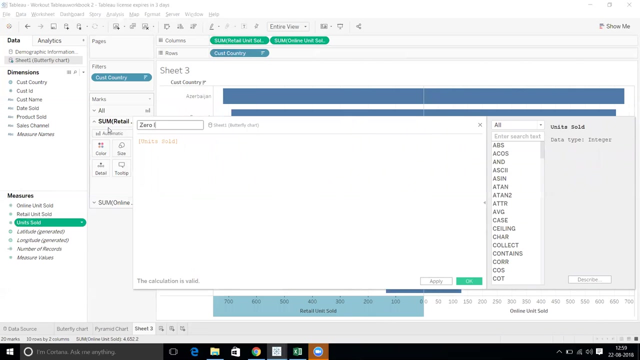 As any descending order, And let's give it make it an entire view. Okay, so now I need to bring this country in between this. Okay, so for that we need to create an axis. I can name it as like zero Right, zero line. 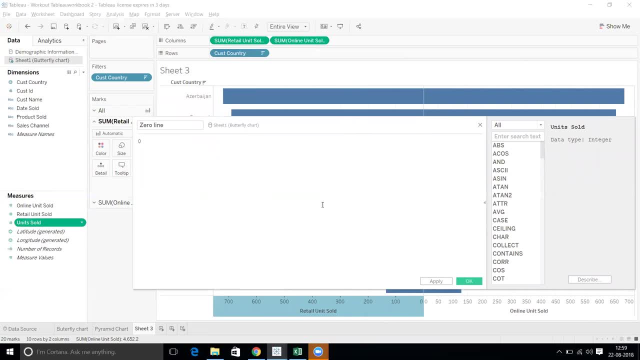 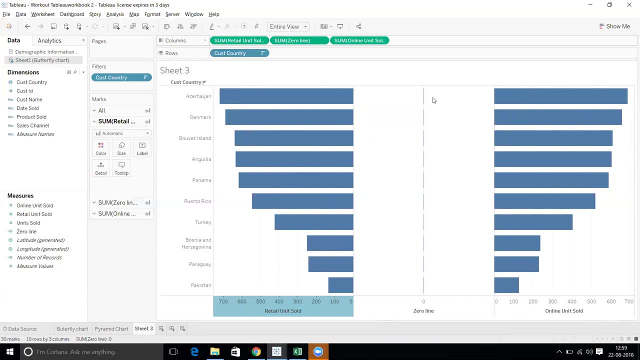 Zero. Okay, just take in between this. Yes, So now we can take the labels here. So in the zero lines, take the customer label over here and go to label formatted to make it center. Okay, so this is it. go to label and make it text, okay, so that the line will be removed. okay, go to text now. 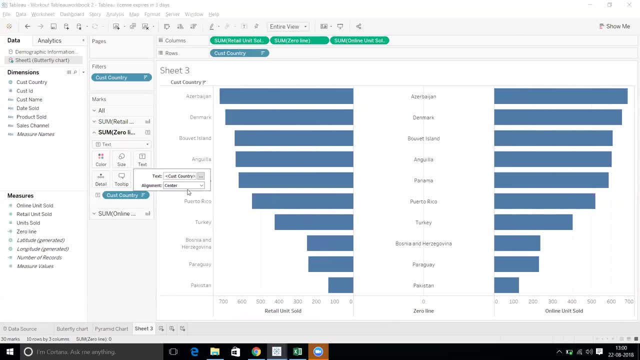 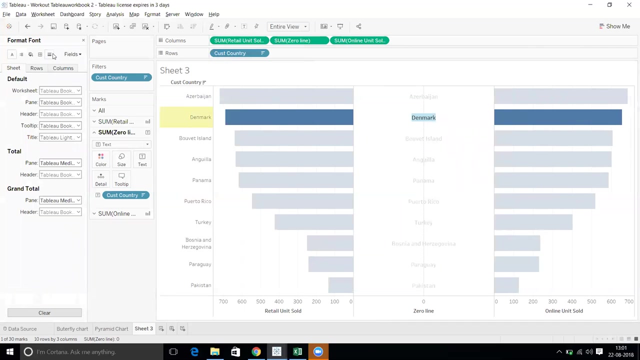 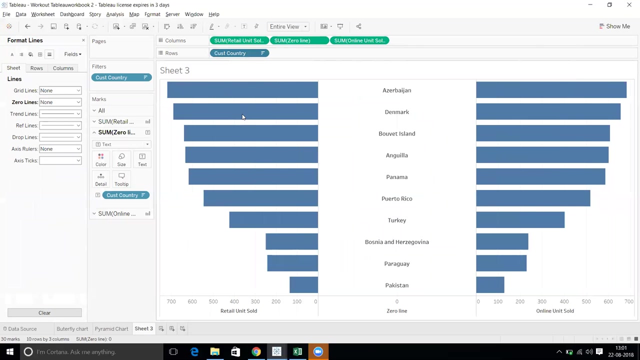 and keep this center and middle. okay, it's too little formatting, for this will carry increase to 10 volt. okay, so fine. so now let's remove the grid lines in between the. so there's a line, actually the lines, zero lines. okay, fine, okay, so let's hide this part as well. show headers. and now what we can do is we can color this. so. 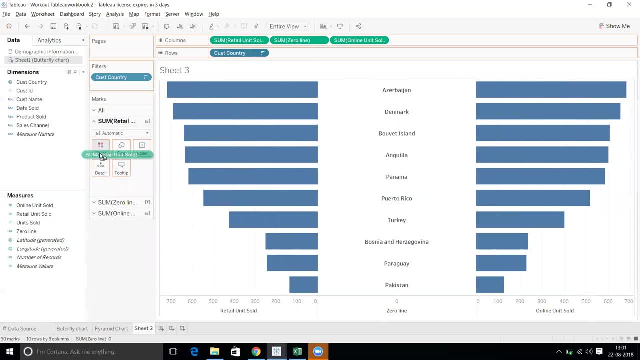 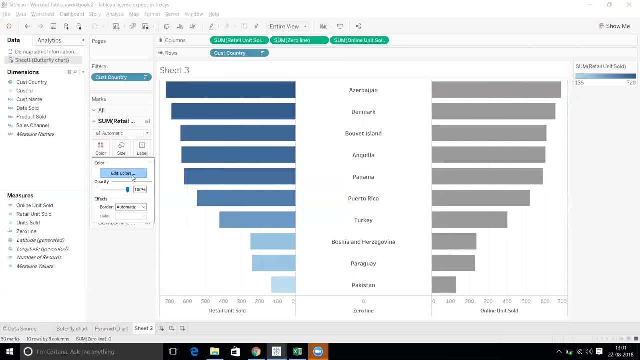 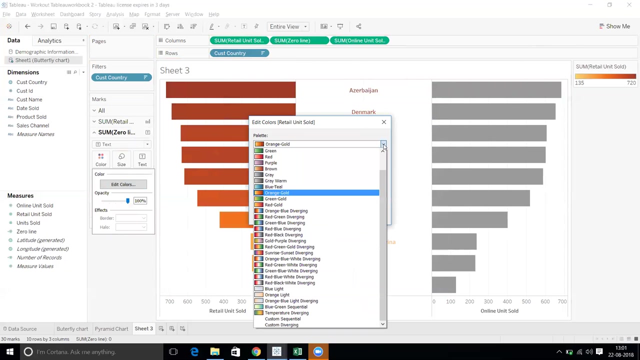 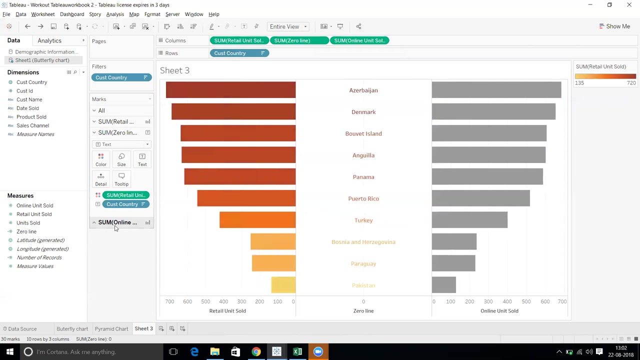 for the retails: drag to color, edit color. I'll take orange gold and retail one is again. we'll take two colors and now edit color and, like green gold, take it to here you. okay, we are like to zero lines, we'll just remove this. okay, all line from here. edit color.